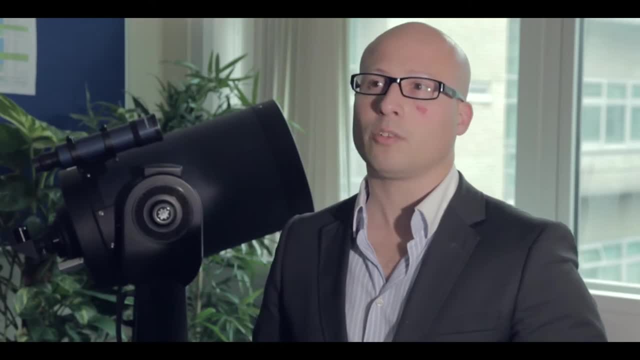 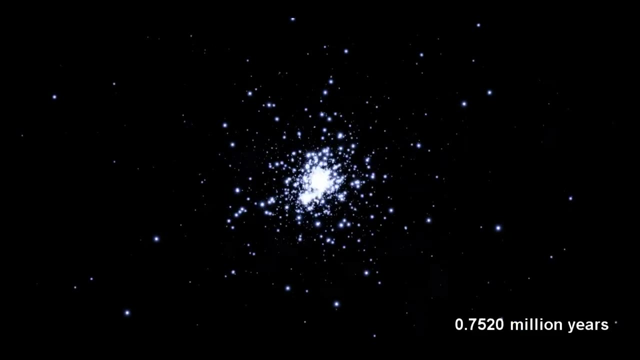 as a whole formed. It allows us to peer into the past, try and understand where we came from and look into the future. what's going to happen to us next? It gives you a lot of skills that you can apply in your further career, even if you 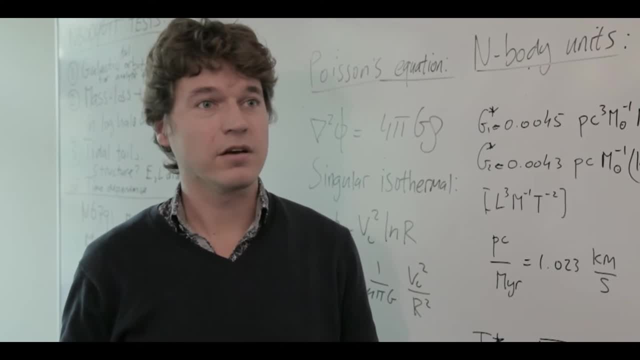 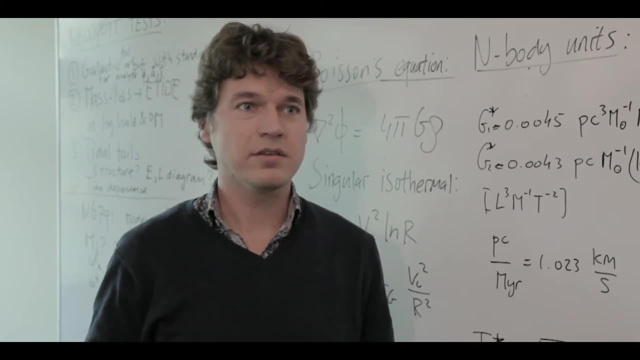 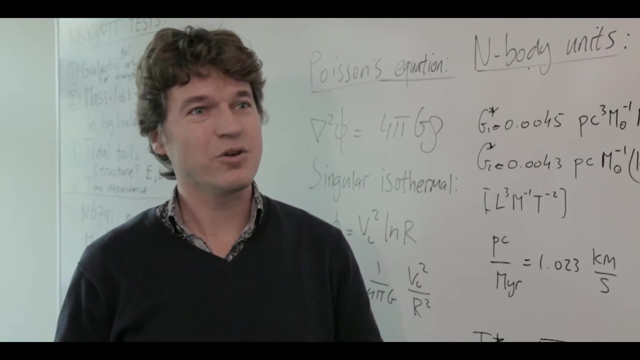 decide to leave astrophysics as a research career. For example, you learn how to deal with large data sets, you learn how to deal with computers and programming, statistical analysis, et cetera. But I think, foremost, the most important part is the fascination. You need to be curious. 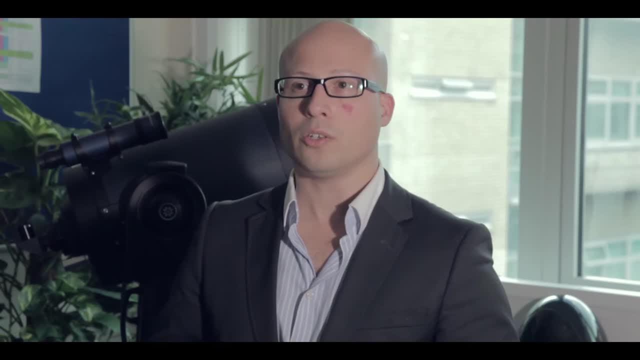 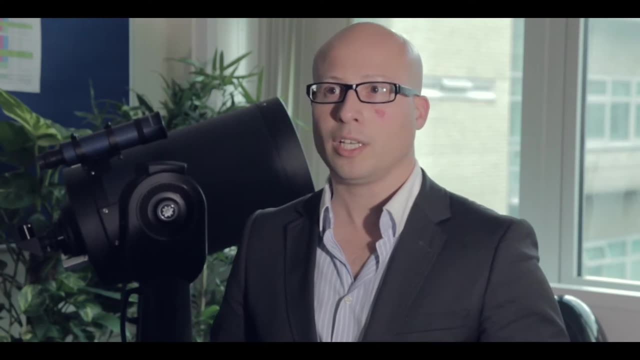 about the universe and knowing how it works. You get a chance to learn physics as a whole, and that comes with a whole host of useful numerical and problem-solving skills that will stand you in good stead whatever you choose to do after your degree. 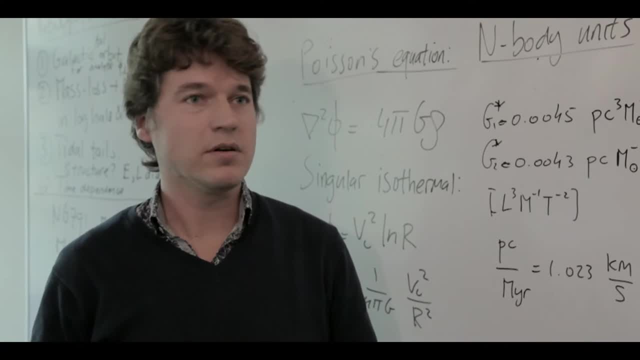 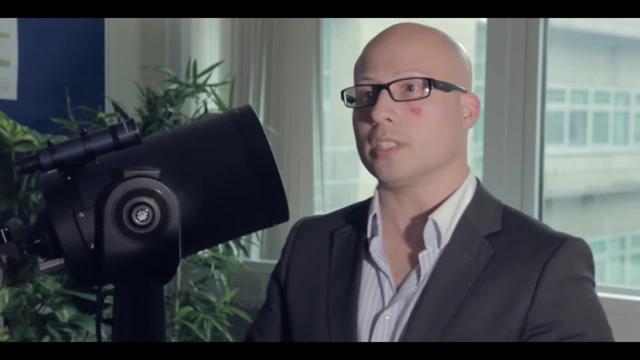 Given the UK's involvement in large astronomical projects, it is only natural that a university of the size of the University of Surrey offers astrophysics as a course. We have an established world-leading space, We have a space centre that specialises in building nanosatellites, and we also have 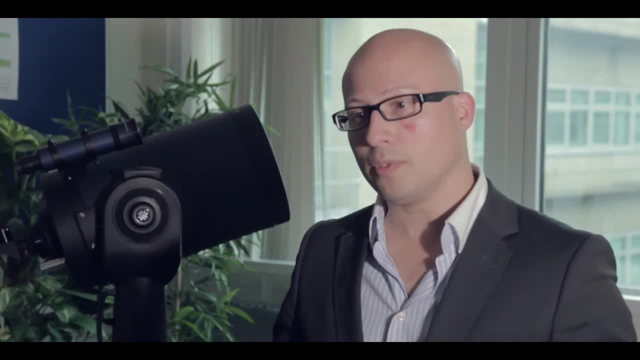 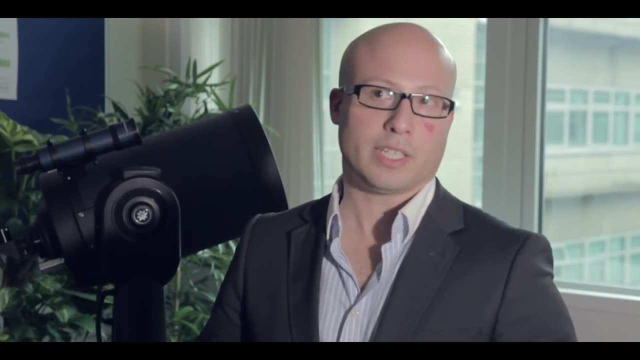 a very strong physics department, So it's quite natural to fill in the gap between those two activities and have a dedicated astronomy group. The other reason is that the UK is a major player internationally in astrophysics research, and Surrey are excited to be a part of that. 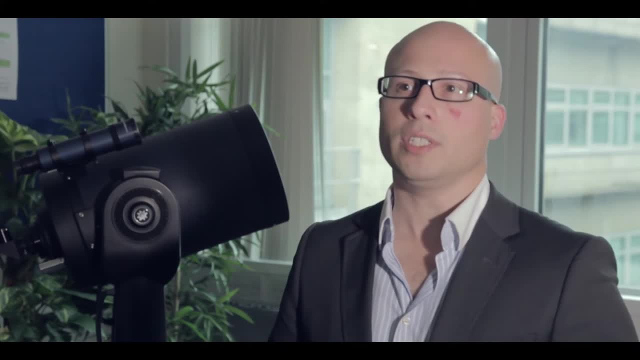 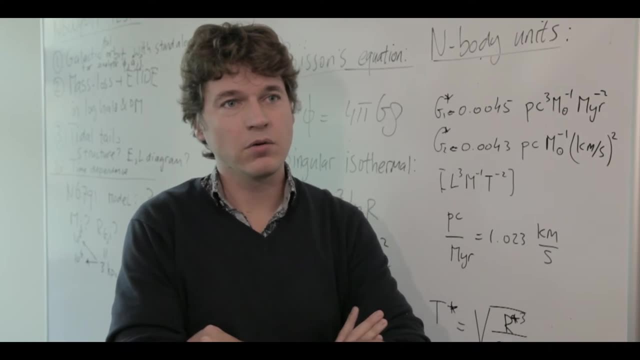 And I think, finally, it allows us to offer greater breadth and diversity to the undergraduate students in what they get to study here, and we're really excited about that. So we are currently developing a whole set of projects. We are currently developing a whole set of projects. 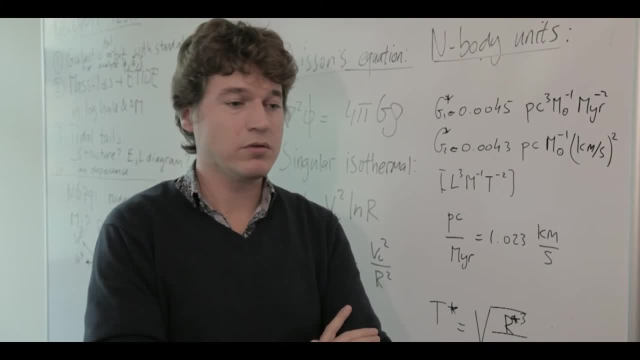 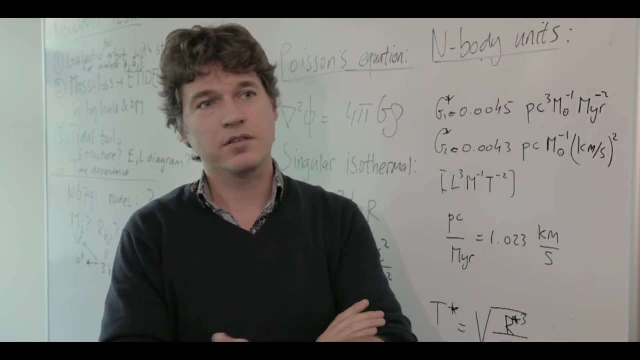 So we are currently developing a whole set of projects. We have a whole series of facilities which we use for our research and will also be usable for the students that enrol in the programme. So, for example, we have a supercomputer centre which has several graphics cards involved. 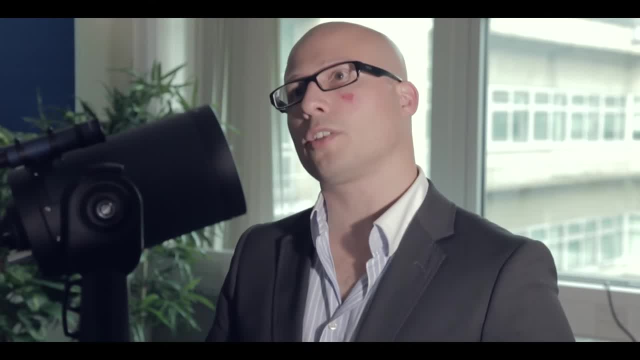 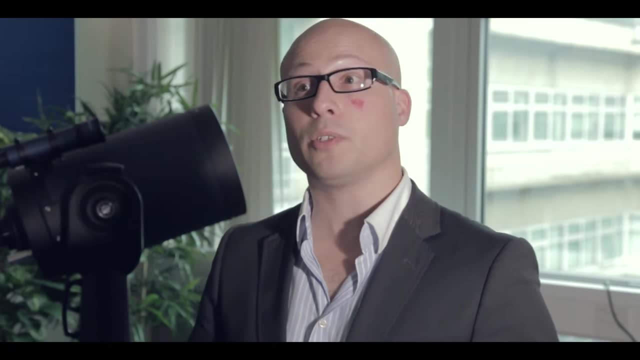 for modelling gravitational systems, And we're also building a teaching telescope here on campus that will give the students the opportunity to have a first-hand observational experience, And the kind of telescope we're going to build is really a scaled version of the very largest telescopes in the world. 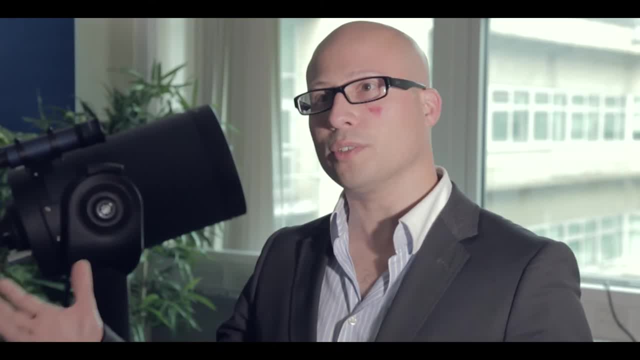 So what they learn here is directly transactional. So what they learn here is directly transactional And the kind of telescope we're going to build is directly transactional. And the kind of telescope we're going to build is directly transactional And we're going to have a very well-designed, highly-transferrable to the real professional. 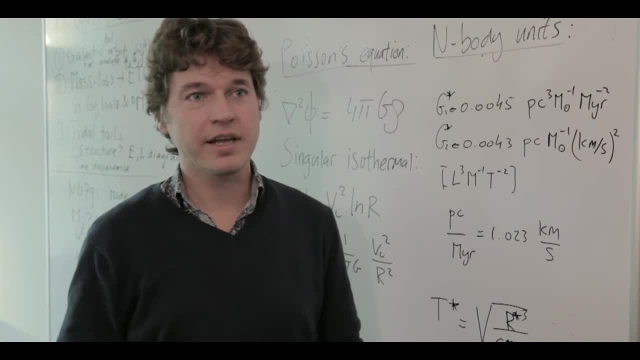 astronomical world And we're going to have a very well-designed, highly-transferrable to the real professional astronomical world. So my research focuses on the dynamics of stars in very dense stellar systems and these we use to understand the origins of our Milky Way. 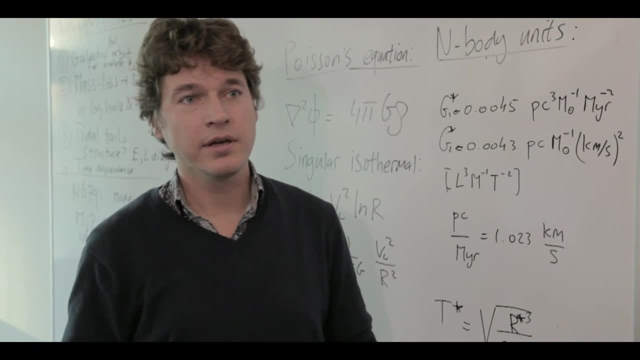 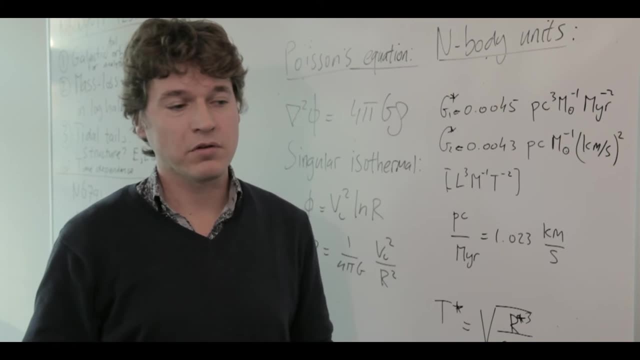 They're formed very early on in the evolution of the Milky Way And we mainly focus on the computational aspect of solving the laws of gravity. This is Newton's law for many, many particles, And we use special hardware for that, like these graphics cards which were originally 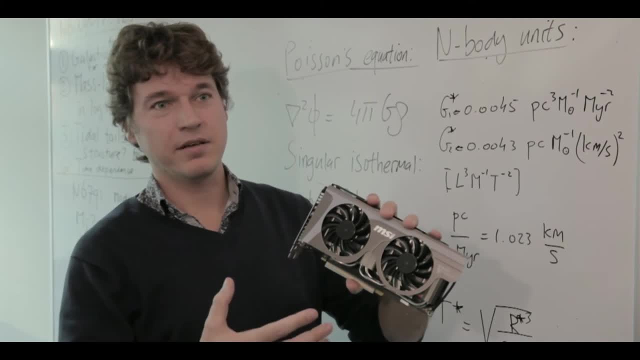 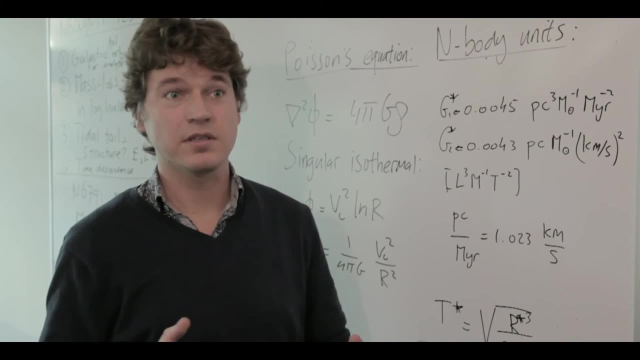 developed for computer games. So they solve basically 3D images and where you can move through, But they're also very suitable to do large-scale simulations of gravitational systems. So my own research is focused on dark matter and this is an apparently invisible substance. 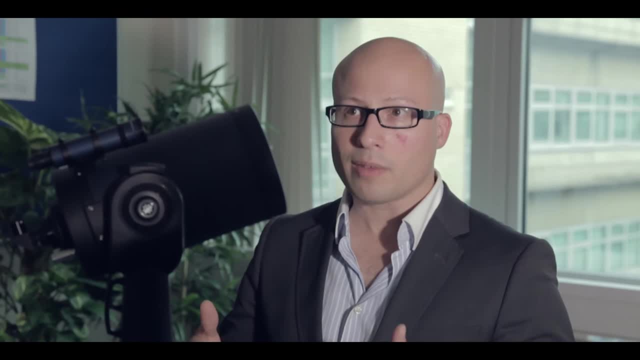 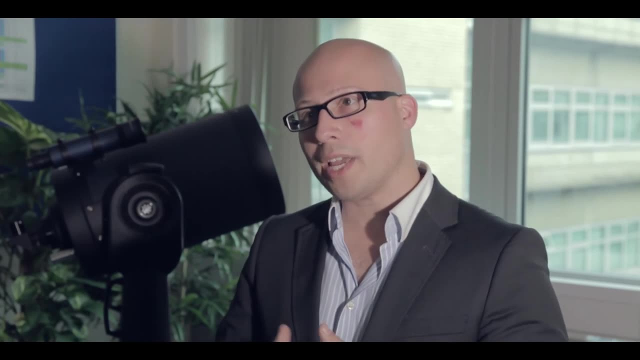 that we think fills the whole universe. We know about it only through its gravitational influence. It's the glue that binds galaxies and clusters of galaxies and the universe as a whole together, And the way in which we probe this dark matter is exactly through its gravitational influence. 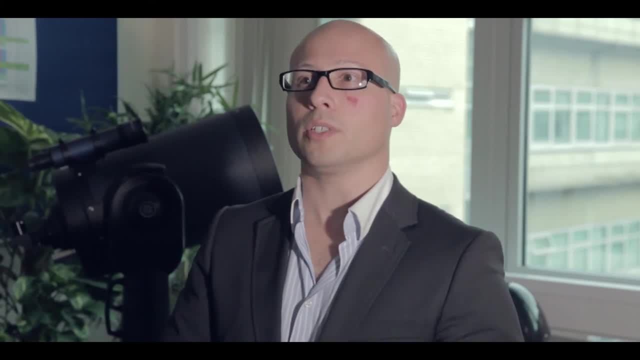 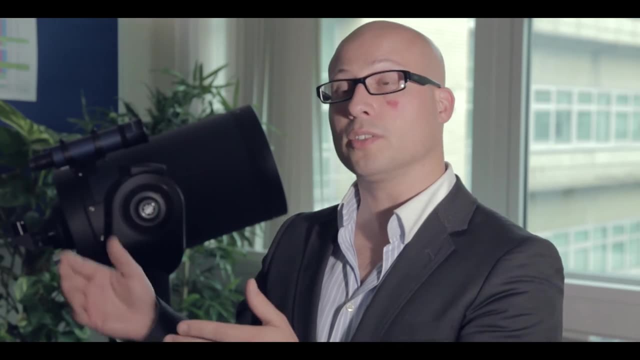 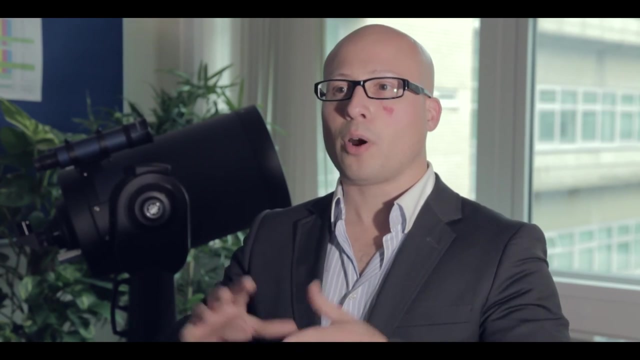 So we run massive computer simulations of the universe, assuming something about the nature of dark matter, And then, by comparing the results of those simulations to detailed observations, we can constrain or even rule out some of these dark matter models. And in fact that pretty much encapsulates our prime research goal for the group as a 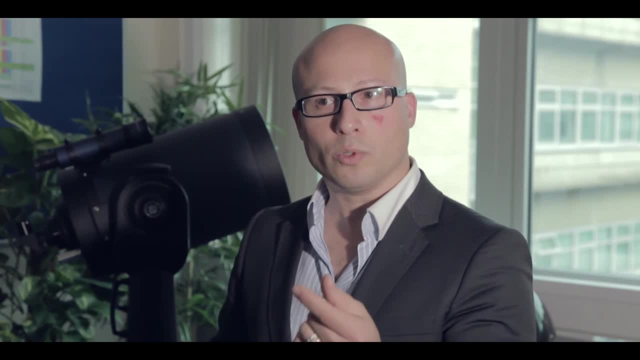 whole is in multi-scale simulations from the very small star-forming sites all the way up to the universe as a whole. The real excitement, I think, is to be able to teach the students from the very beginning, from the very beginning to the very beginning, to the very beginning, to the very beginning. 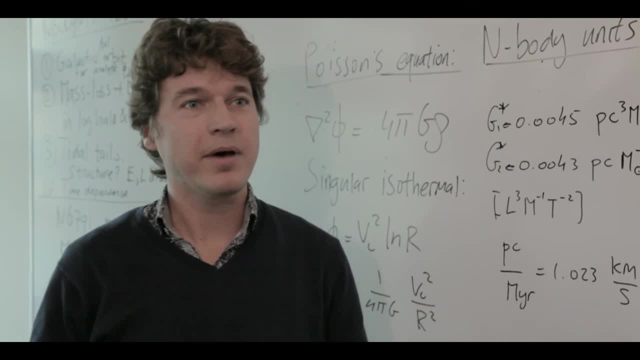 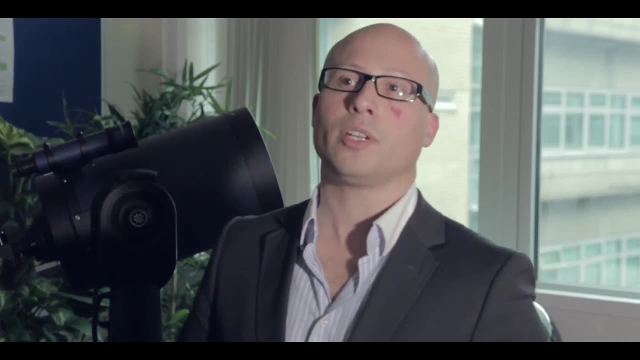 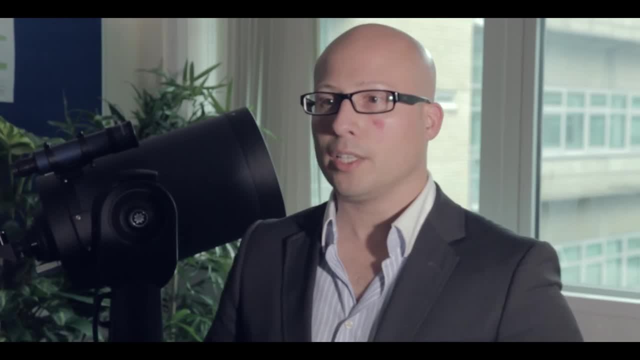 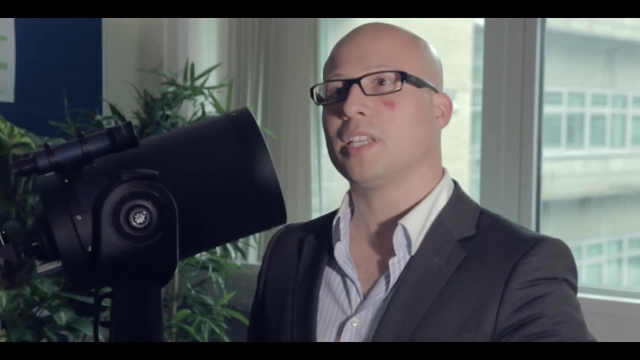 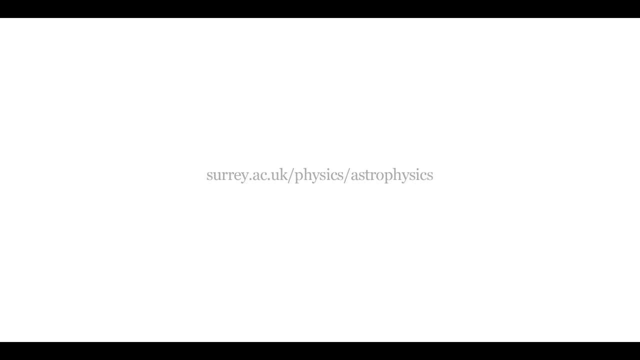 go on in the very best that make it through to the master's level, to being researchers in our field, And I'm looking forward to meeting the next faces that will shape the new discoveries ten years down the line. Thank you, Thank you. Thank you.